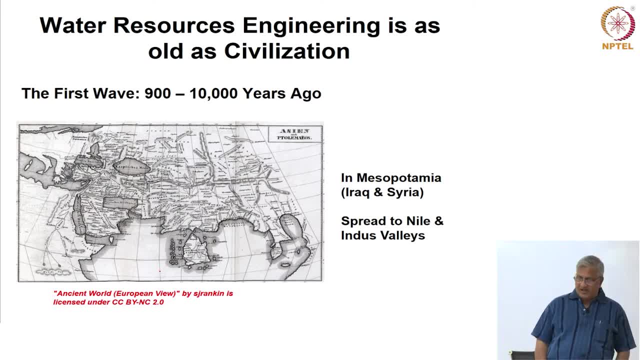 particularly on the banks of rivers or river valleys. They say that it started in Iraq and Syria and Mesopotamia and then slowly it spread to Nile Valley and Indus Valley And you all know about Indus Valley civilization and in fact about Nile. So water resources. 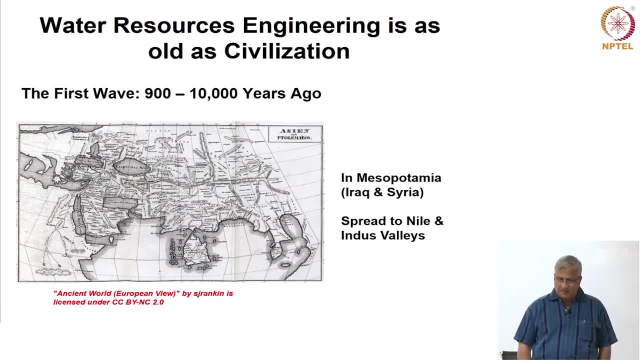 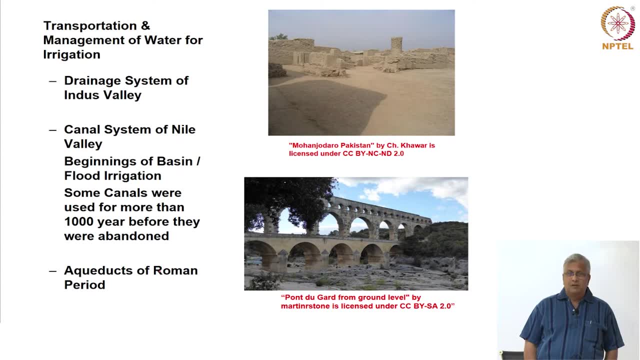 engineering is as old as that. Like, for example, when people settle down on the river valleys, they needed transportation In management of water when they started agriculture, you need that for irrigation, Like canal systems of Nile Valley. that's basically the beginnings of what we call. even now we 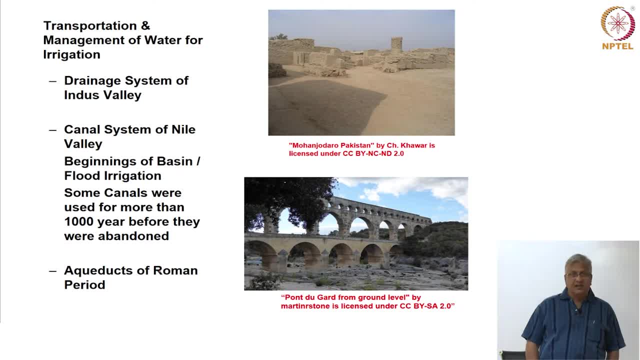 practice in many parts of the world called flood irrigation or basin irrigation, And some of these canals where they used to divert the water from Nile to these fields or tanks, Those canals are more than I mean. they were used for more than 1,000 years before they. 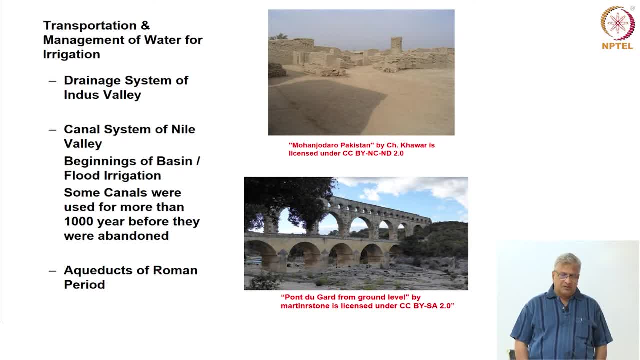 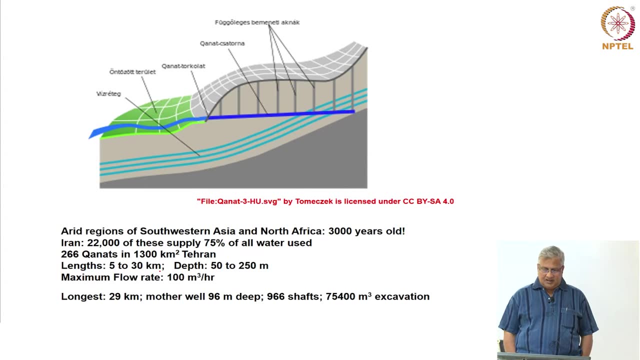 were abandoned, And we all know about the drainage system for wastewater in Indus Valley, and we also know about aqueducts of Roman period. There is another thing called canards. These are basically used in arid regions of southwestern Asia, Asia and North Africa. these are about 3,000 years old, and then they are still surviving. 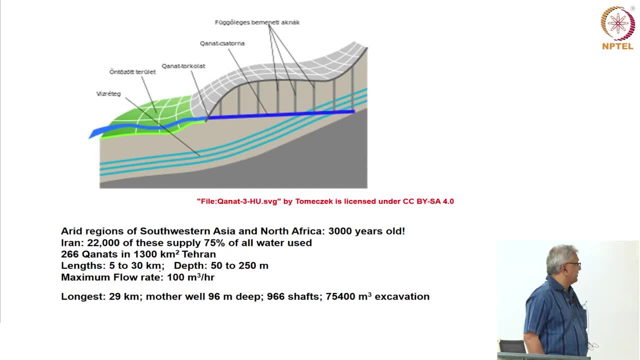 Basically, Iran has like 22,000 of these, supply 75% of all the water used. What they do in these canards is basically, whatever the water that is falling on the mountains or the hills, that water seeps into the ground and then that blue line: there you. 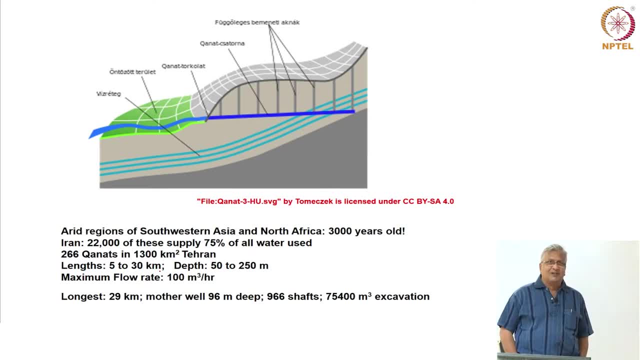 see, This is actually a tunnel dug into the mountain from the base of the mountain and they capture the water and the water flows in this tunnel and then comes out of the mountain and then it is taken through canals to wherever they want to use this water. 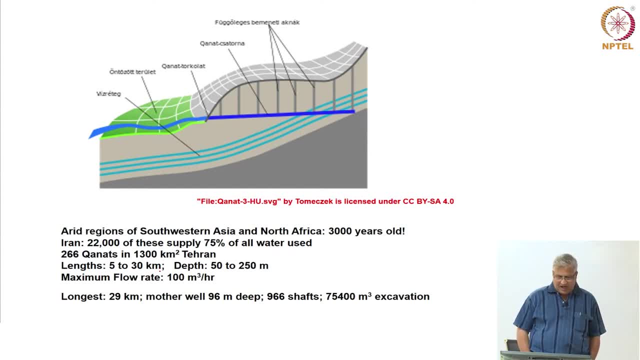 These are called canards, and then they're about 5 to 30 kilometers land, 50 to 250 meters depth, and sometimes they carry as much water as 100 meter cube per hour. The longest is about 29 kilometers. Some of these canals are called canards. Some of these canals are called canards. Some of 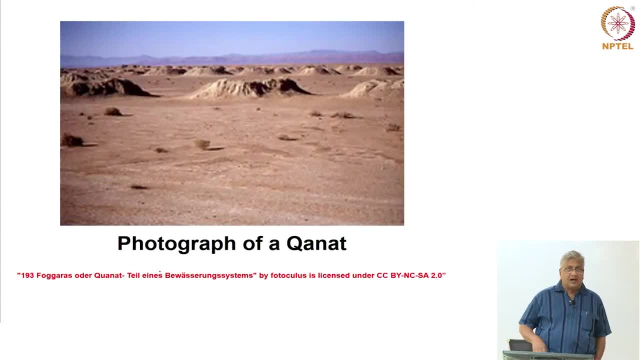 these things are still existing and working fine. Some pictures of these canards from the surface: when you see, that is basically there is a tunnel going underneath and then they have, in fact, manholes and then things like that for inspection of these canards. All this is 3,000 years old, so it's not something that we have been doing in the last few years. 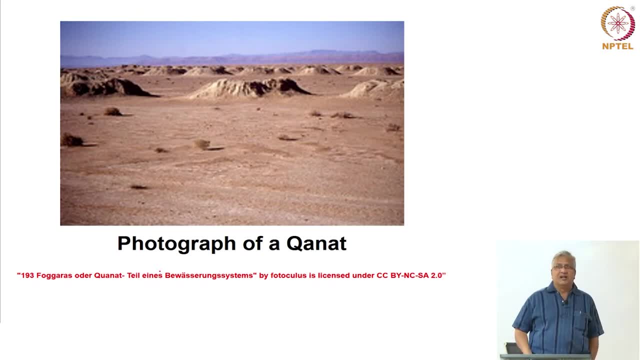 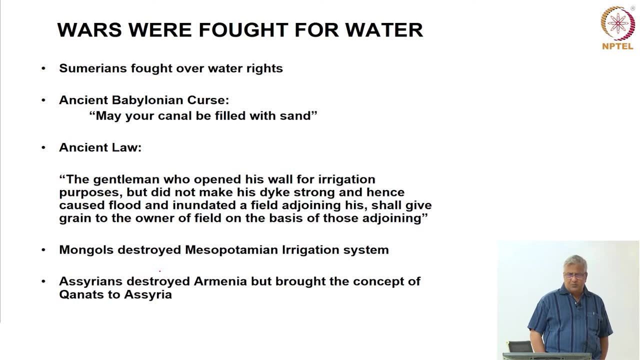 So that's why I say hydraulic and water resources engineering is as old as civilization. And another important point, Another important thing was wars were fought for water. Like Sumerians, they fought over water rights- Who should get how much of water? And you all know we still fight for water. 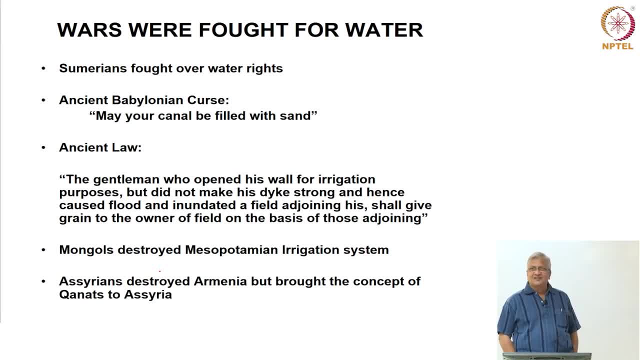 within the states, within the countries and so on and so forth, Like there's an ancient Babylonian curse like to say: may your canal be filled with sand. What it means is it's like cursing somebody, a society. If your canal gets filled with the sand, then you won't. 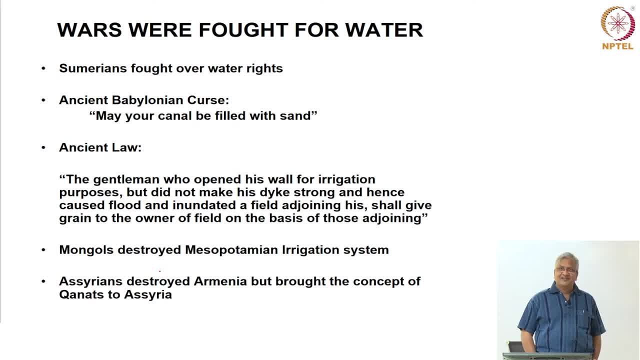 have water for irrigation, and then the economy will be bad. And then laws were formulated or policies were framed, Like gentleman who opened his wall for irrigation but did not make his dike strong and hence cause flood and inundated a field adjoining his. shall give 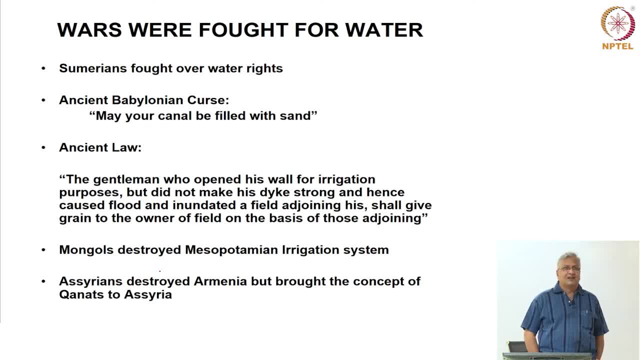 grain to the owner of field on the basis of those adjoining. That means people were aware of water law. Again, it's not that something new that we are doing now. Mongols destroyed Mesopotamian irrigation system. It's like these days when there's a war one thing. 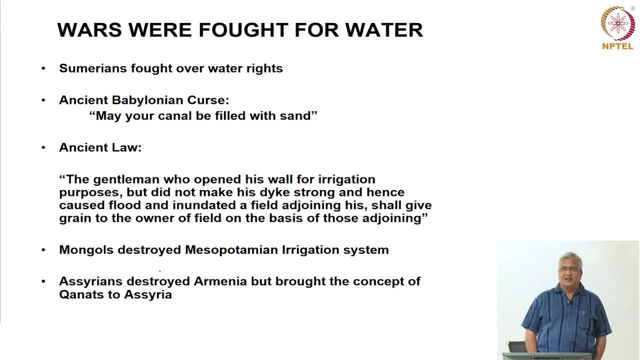 they do is they will attack the- you know economic or infrastructure installation right to keep the- I mean the enemy's economic system- down. So they were actually doing that for irrigation systems. Assyrians also destroyed Armenia, but then when they went to Armenia, they found that this that I was discussing about few minutes ago is something pretty. 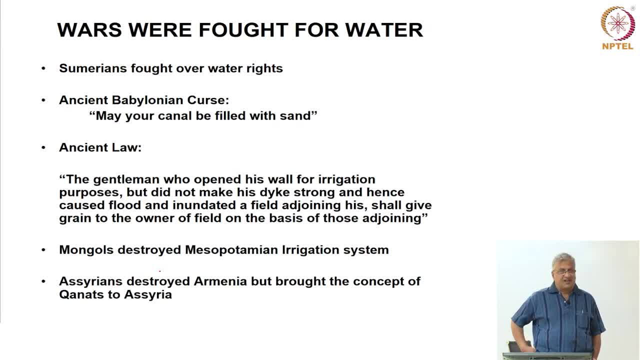 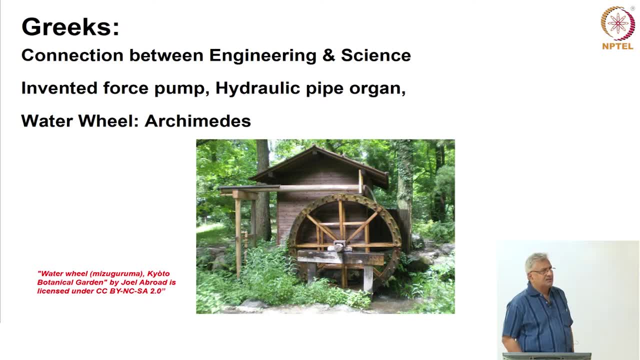 good, So they destroyed them. but then the concept of canards: they took it to Assyria. And I'll jump, of course, Greeks in the western world. The Greeks were the first who got the connect, the link between engineering and science. They said, okay, you would, you've been doing. 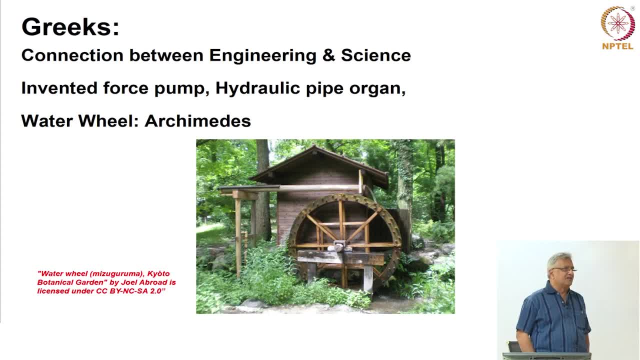 all this engineering but we need to understand the basics of hydro science. So they said that's very important. So and then they invented- They said force pump, hydraulic pipe, water wheel. I mean, Archimedes has invented water wheel and how to lift the water and use for many purposes. So I just jumped from there. 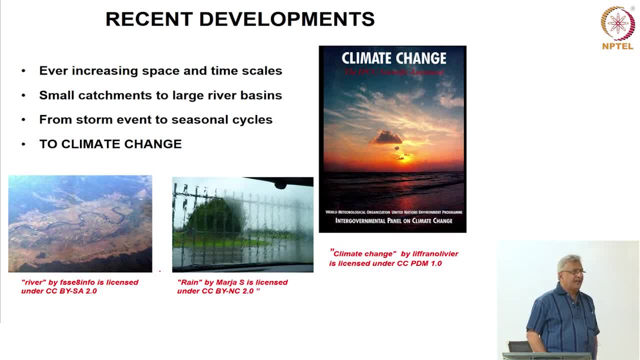 to what stage we are in, like recent developments. For example, presently we are as hydraulic and water resources engineers. We are concerned with ever increasing space and time scales. When I say spatial scale, you can go and then say that I'm interested in what happens in, let's say, IIT Madras lake. How much of water is? 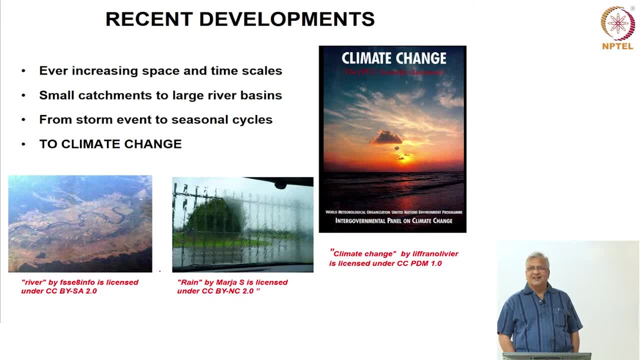 there. How will I utilize this? That's the smallest scale that I can start with, And then I can also discuss about what happens to the water resources, let's say in Ganga river basin. So we say small catchments, we can think of studying, We can think of the. 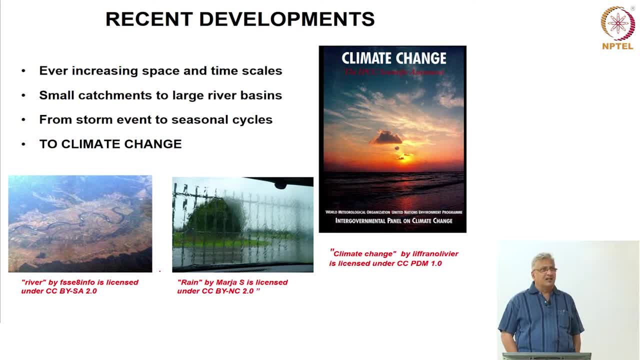 hydrology or water resources in, let's say, IIT Madras campus. starting from there We can go and then look at what happens in, you know, a big river basin, And then we can start from a storm event. Let's say there is a 24 hour, 100 year rainfall, Like a 100 year rainfall. 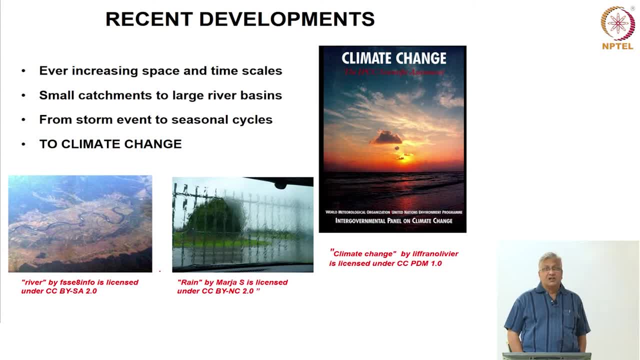 may be, like you know, 300 mm of rainfall coming in 24 hours in Chennai in 2015.. What kind of floods it caused. So that's the kind of time scale. So that's the kind of time scale. This may be few hours, or, and then we can go to what happens to the water resources. let's 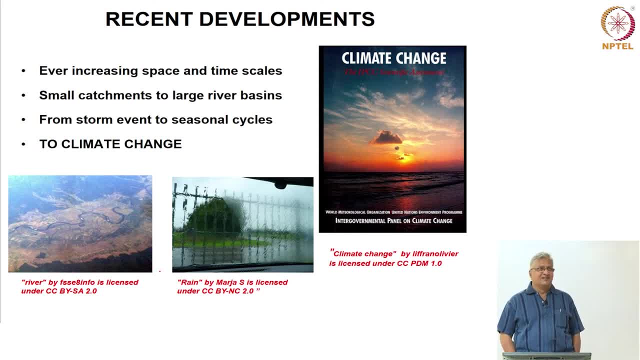 say in Chennai basin or in whole of India, if I increase the spatial scales over a season or over a year, Because we have, let's say, what happens in monsoon season, Or we can increase the time scale to what we call the climate change, Because the climate change 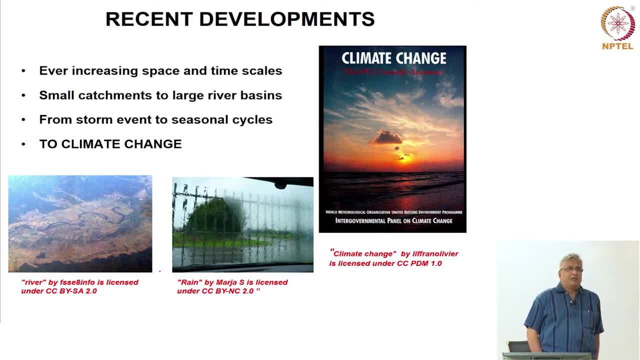 is imminent, And in another, Let's say from 2050. if I design something now, Let's say water distribution system, I would be designing for 30-40 years to work. I mean it should work for 30-40 years And 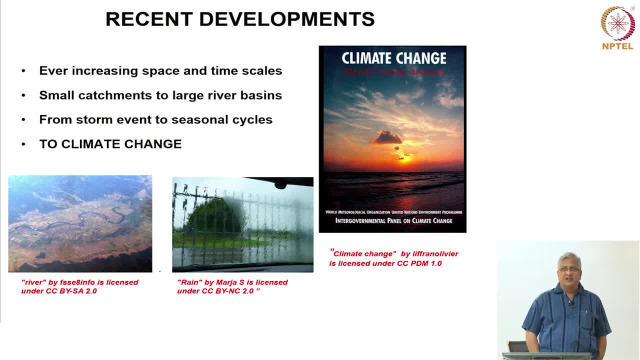 from now, in 30-40 years, what would be the climate, What kind of changes that would occur to the climate And what would be its impact on what I am designing now? That would be, you know, a very crucial thing. That's why I said: 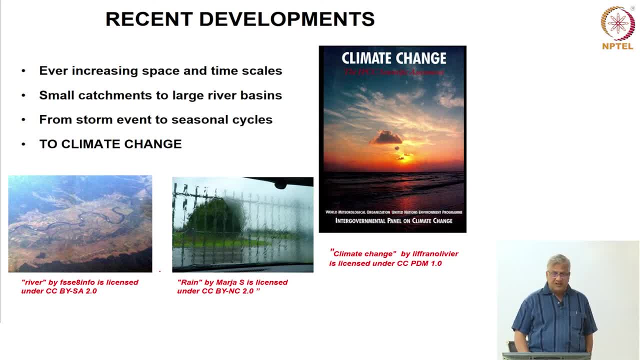 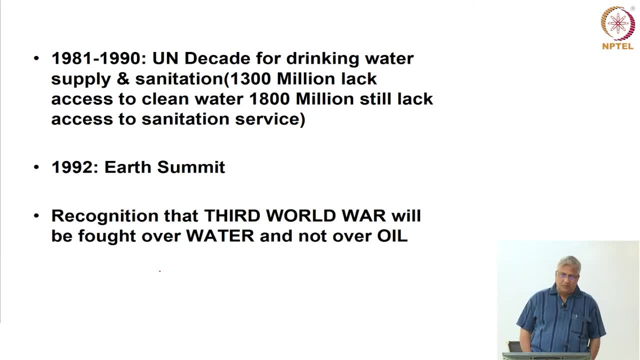 I think the recent developments have been in direction of ever increasing space and time scales. How water resources is engineering? How important water resources is engineering is, let's say, 81 to 1990. United Nations declared that for a drinking water supply and sanitation. because 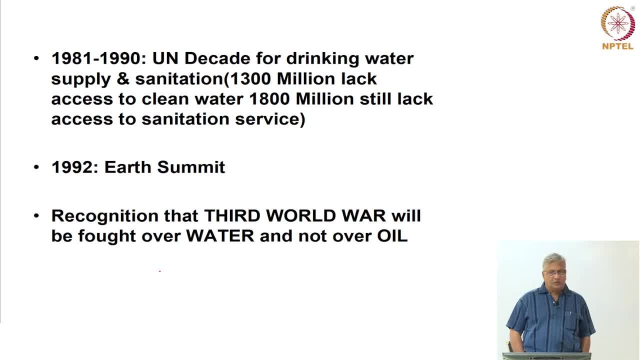 millions lack access to clean water even now all over the world, And millions still lack access to sanitation service, So I think this is something that should be considered in the future. Thank you, So you would be surprised to know that even in India, now, in 2019, only 30 percent of whatever 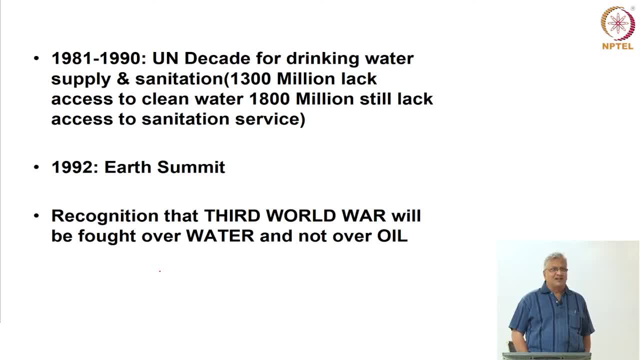 the waste water that gets generated is actually being treated before it is let into the environment, And what kind of you know environmental degradation it would cause, what kind of pollution it would cause to our water bodies, what kind of stress we would have for finding the sources. 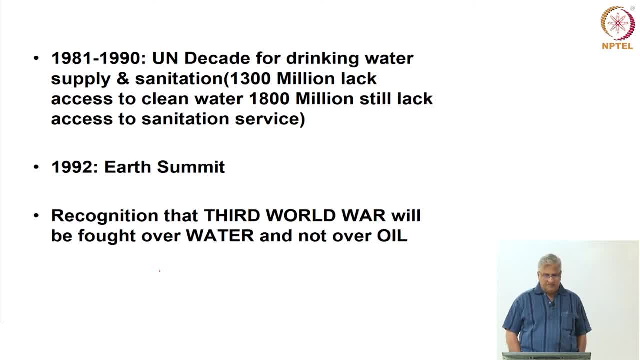 for drinking water because of this pollution. you can imagine, In 1992 we had Earth Summit and of course the society, the world at large, has recognized that third world war will be fought over water and not over oil. In this context, I would like to say one good news is we do. let's say, India shares its 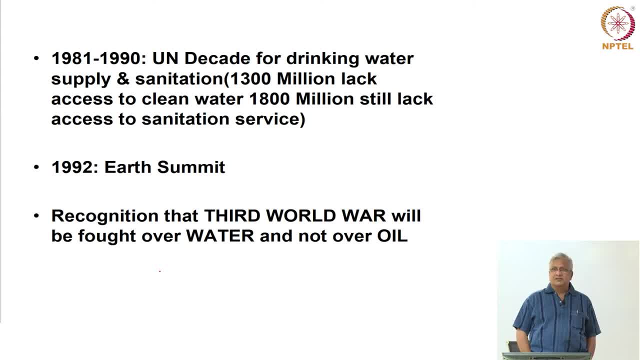 waters with the neighbors, for example Pakistan, The water in the Indus river, and we have an Indus river treaty which came into existence in late 1950s at the insistence of World Bank. at the time World Bank was giving the money and then they said: you two countries should sit together and develop water resources which 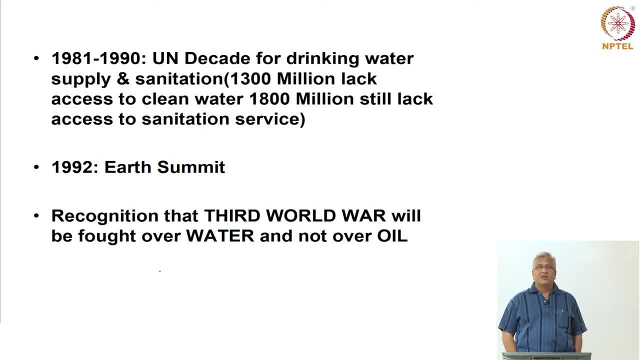 is a common resource for both of your countries. So you have to come to an understanding in a treaty and this particular treaty actually survived all the you know, wars we had with our neighbors. That's what we do understand. everyone understands that water is important and another development: 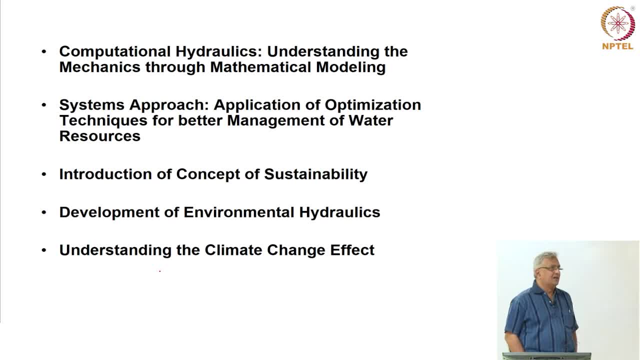 that has taken place in recent years, probably with the advent of computers- once the computers came in late 1950s and 60s- and computational technology has been developed, we have developed what we call computational hydraulics, which is basically understanding the mechanics through 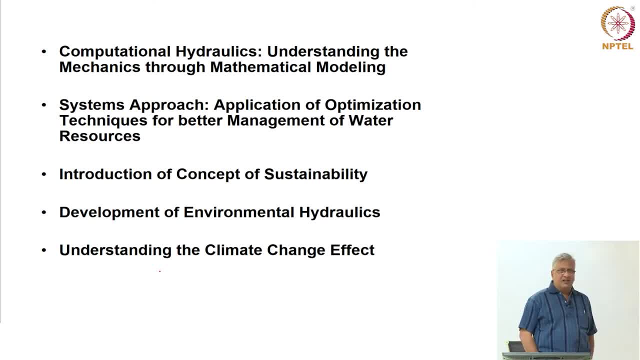 mathematical modeling. We need to, we don't have any other go. but we need to understand the flow of water, particularly when you talk about very large spatial scale and very large time scale, and we want to see what is its effect in the future, and so on and so forth. 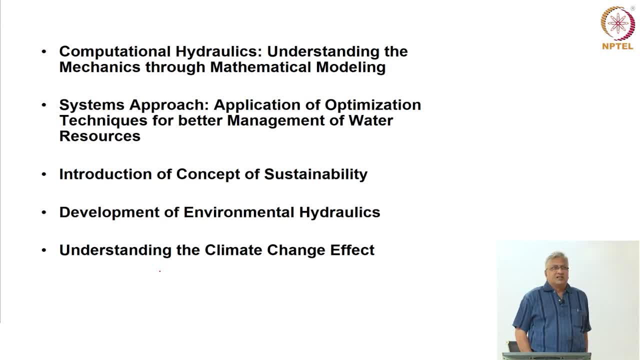 We will not be able to just base our decisions on observations, the previous observations, the past observations, because we have to go into the future and then we also cannot effort to make so many observations. let's say, Ganga river basin. I want to understand the flow. 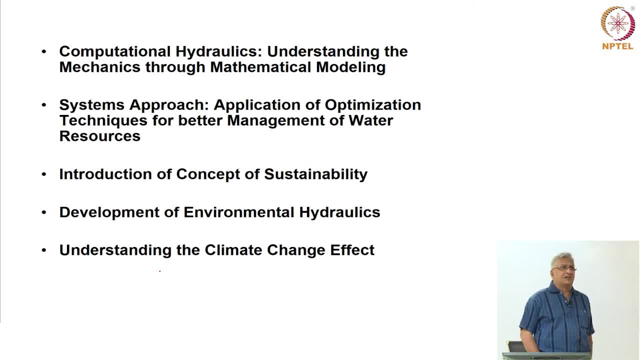 of water, existence of water where it is going from one location to another location. I need to have some kind of a model, a mathematical model, which I use for taking the decisions. So computational hydraulics, that is, understanding the mechanics through mathematical modeling. 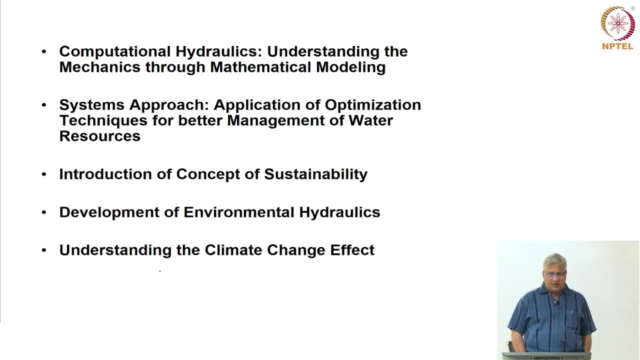 has been a focus of attention in the last 4 decades. another thing is what we call the systems approach. That is, whatever we do to the water at one location, you may have a consequence of it at a later stage, or maybe at a later time. 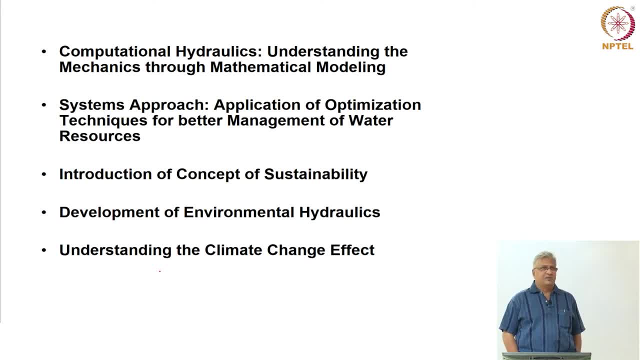 Let's say I was telling in my other class- I think most of you- I don't know whether you have attended or not- ID 1200,. if you build a dam, it will have many, many consequences and some of these consequences may be felt, may be hundreds of kilometers downstream of 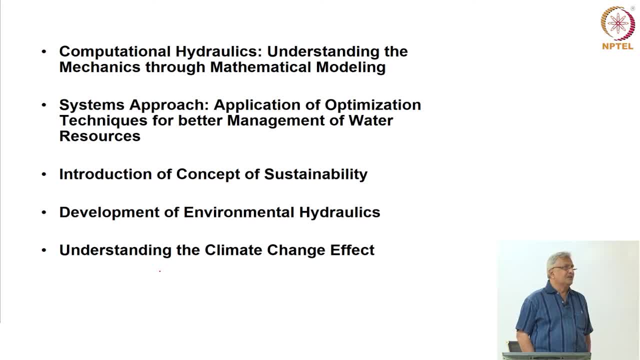 the dam and then maybe after 30,, 40 years or 50 years. So you need to get a systems approach. you have to see the interconnections. and another thing is you need to have optimization techniques for better management of water resources. So that has been another what you call advancement that has been made in hydraulic and water. 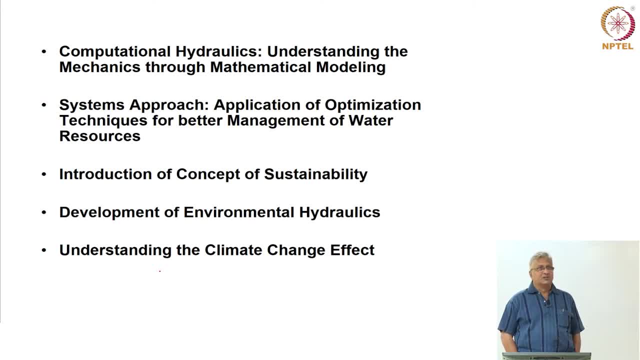 resources engineering. We also, of course, introduced the concept of sustainability Now 2015, on-map. We have developed the concept of sustainability Now 2015, on-map. In other words, we have sustainable development goals, which was follow up to our millennium development goals. 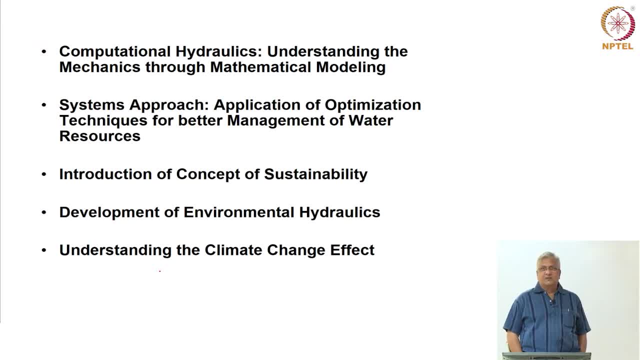 So water resources also have to be developed with the concept of sustainability in the background. Another important this thing that has been made is in terms of environmental hydraulics, like we talk about eco flows in rivers, how much of flow that we have to leave in the 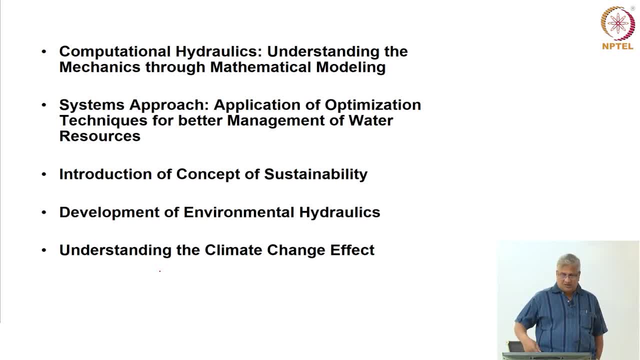 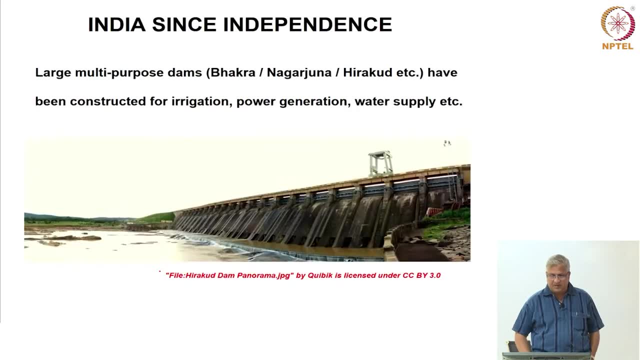 river. You can see this in the background. The ecology is not disturbed. and then, as I mentioned already about the climate change effect, is also important. Since independence, India has made lots of advance in terms of water resources, like we have built. right after the independence, we started building dams because we needed to. 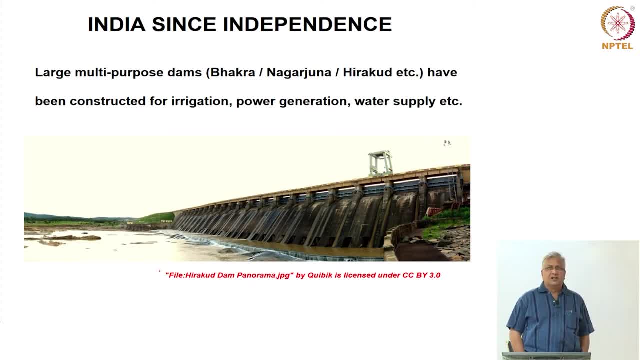 get food security. We went through lot of famines and then we needed to get food security. that means we had to increase our irrigation potential and food production. large multipurpose dams were built, like Bhakranangal dam, Nagarjan Sagar dam in Andhra Pradesh and then Hirakut dam in Orissa- the picture that I am showing. 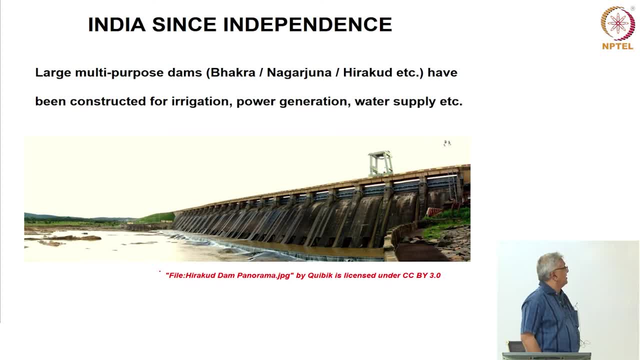 here is actually that of Hirakut dam, the spillway. these have been constructed for increasing the irrigation potential, the hydropower generation water supply, the domestic water supply, industrial water supply- one thing that I have not written here, but it is also. 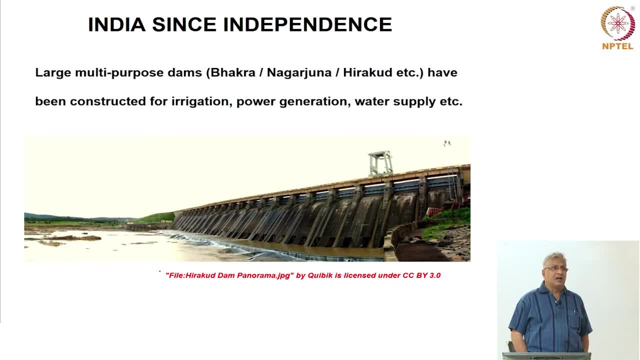 very important, particularly in the context of Hirakut dam, the flood protection. okay, in fact, Damodara valley corporation, that DVC on Damodara river, is also basically a multipurpose. most of these things are multipurpose hydroelectric, large hydroelectric, I mean hydropower. I. 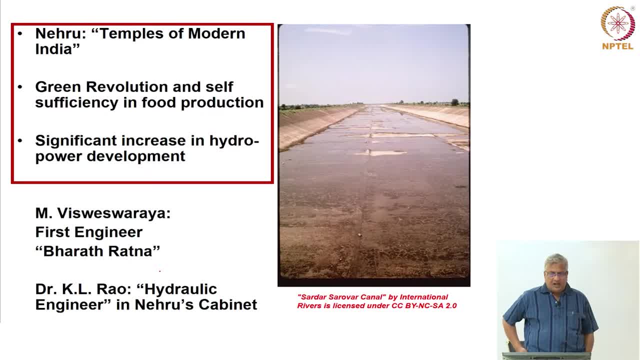 mean hydraulic structure schemes. okay, In fact the prime minister at that time, Pandit Nehru, they called these structures as temples of modern India and they were required at the time because green revolution. they triggered the green revolution and self-sufficiency in food production. because by early 1970s, 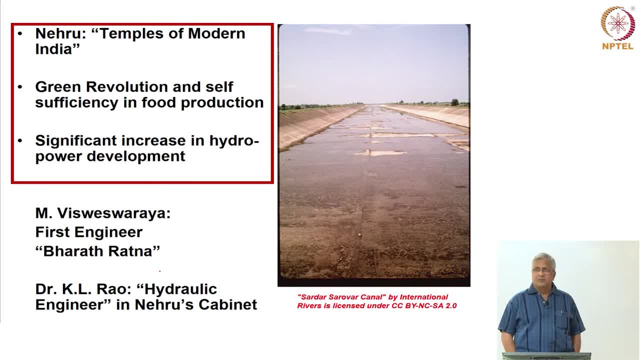 India stopped actually importing the food grains, otherwise we were depending on the other countries. So these are some of the reasons for our food, and there also has been a significant increase in hydropower development and just to tell you how important hydraulic and water resources 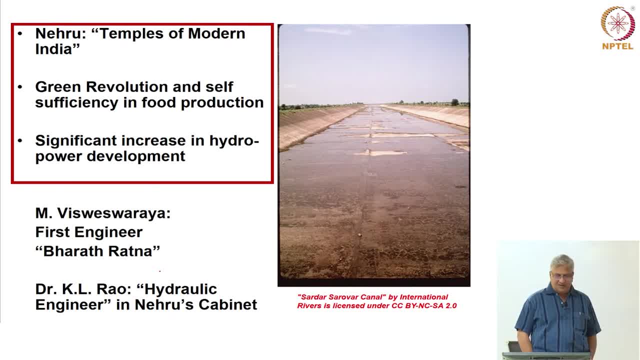 engineering is to the society and to the nation. Moshagundam Visvesariya is the first engineer who was awarded Bharat Ratna and then in fact he was a hydraulic engineer and water resources engineer, And in early 60s they realized the importance of hydraulic and water resources engineering. 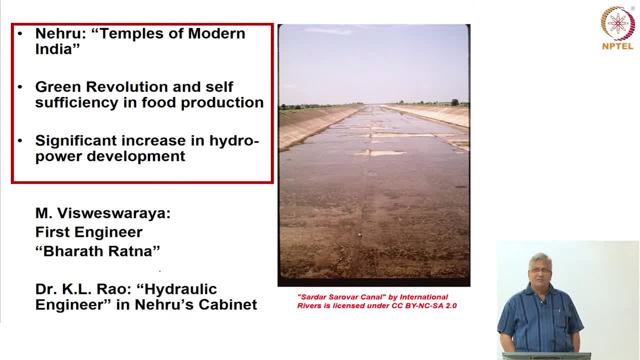 for the development of the society, and Dr KL Rao was actually made a minister. he is not a politician, he is actually a technocrat. and then he was made a minister in the cabinet, minister for water resources. I just to give you an idea about how important these things are and the picture that I show. 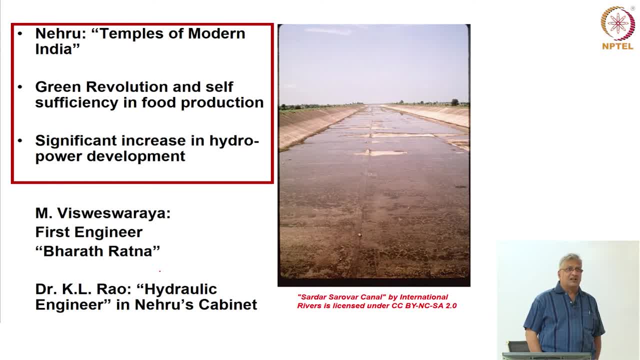 you here about the canal is what we call Sardar Sarovar canal. This is the canal that we call Sardar Sarovar canal. This is the canal that we call Sardar Sarovar canal. This is the canal which takes off from Sardar Sarovar dam in Gujarat and then supplies water. 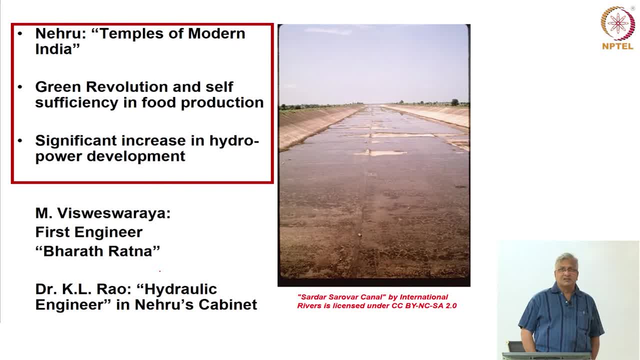 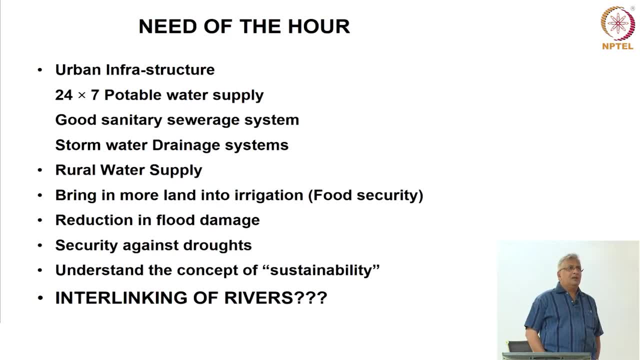 to, you know, very, very water scarce areas like Kutch, and then probably some of this water goes to Rajasthan too. So the need of the hour, why we need to study hydraulic and water resources engineering, is basically one thing that is of importance is urban infrastructure. 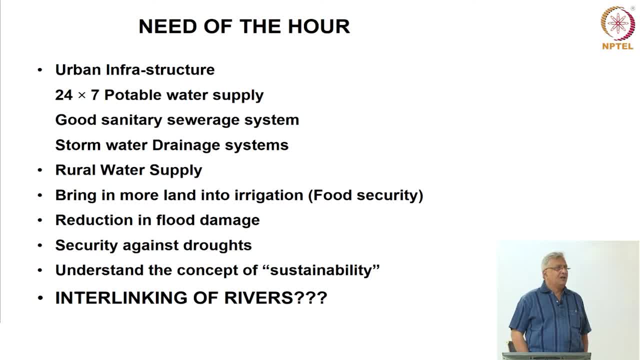 all part of your hydraulic and water resources engineering, and the country needs that too. 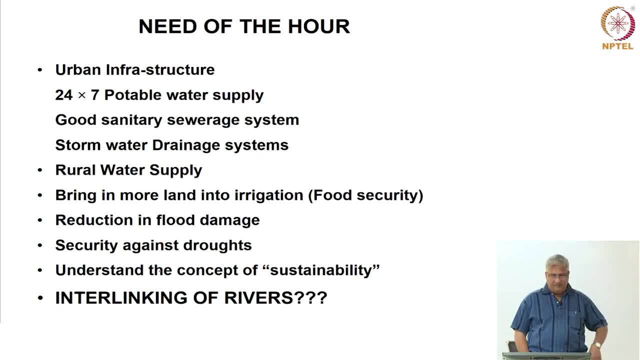 And I already mentioned about rural water supply. and then other one is all these urban infrastructure is always in the news because we have 40 percent of the people living in urban areas these days and of course, the urban population is also going to increase by leaps and bounds in in future. 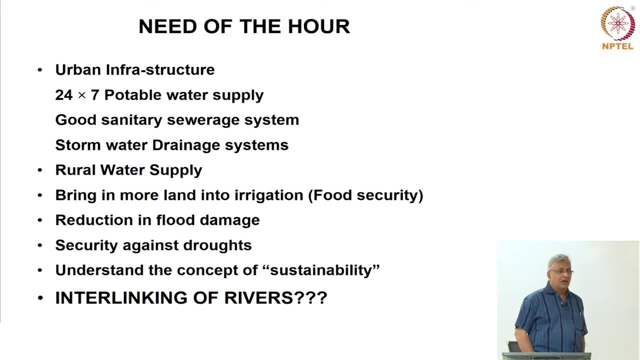 That is why urban infrastructure- I put it at the front before. But if you look at the usage of water, the bulk usage of water, 85 percent of our water resources are actually being utilized for agriculture, Domestic water supply. we use only 6 percent of our water resources. the 85 percent goes. 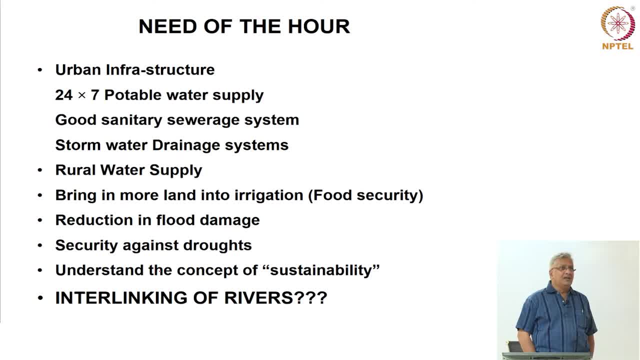 into agricultural sector, And then We need to utilize this water in agricultural sector in a much better way. Right now, the efficiency of water use efficiency in agricultural sector is very low and may be 25 to 30 percent, and we need to increase this water use efficiency to 60 to 65 percent. 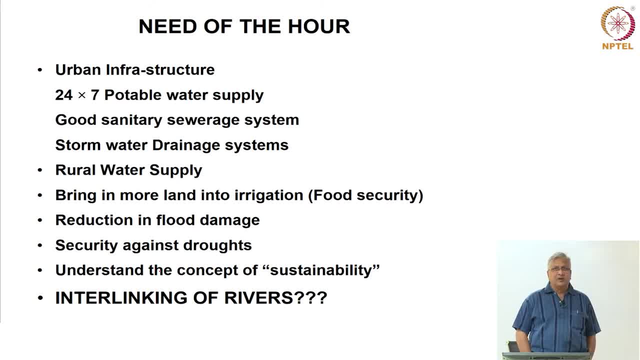 if we want to bridge the gap between the production of food grains and what is our demand for the food grains in the future, for the future population. So this, basically: we need to bring in more land into irrigation and we should get a better ways of irrigating. we should get better returns for every drop of water we use in our agricultural. 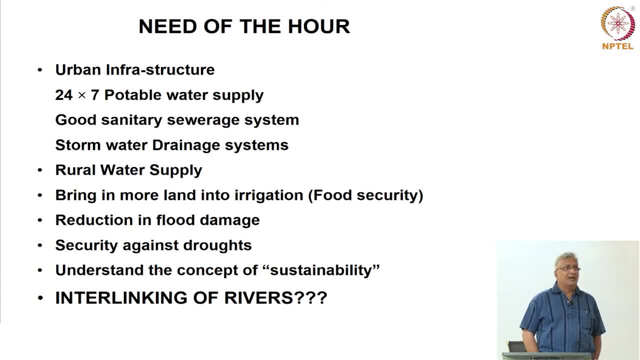 fields very, very important. So there again, We require hydraulic. and so when you say irrigation engineering, it's not just agricultural people but it's to do with water. so civil engineers who have a background or knowledge of hydraulic and water resources engineering will be called upon for that. 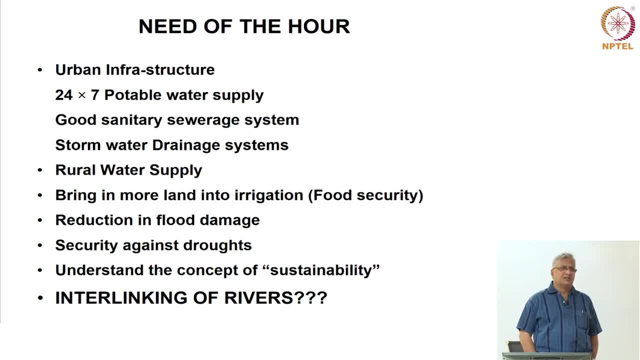 And, of course, I don't have to tell you about the flood damage. For example, 2015 floods in Chennai in fact accounted for 30 percent loss of money of the Entire years, loss of money due to, you know, natural disasters. just one flood in Chennai. 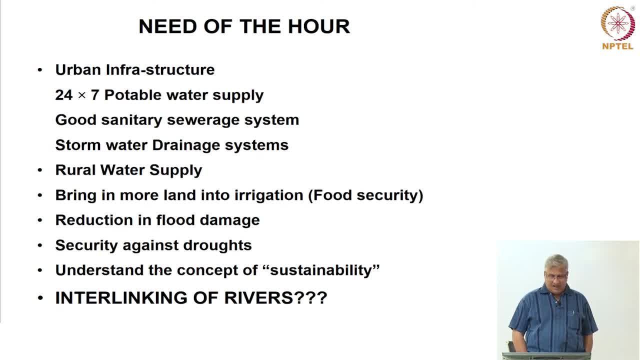 accounted for 30 percent of you know, economic loss and you also heard of the floods in Kerala just last year and floods now. It's irony that in some places you have lot of excess water problem, like floods, and then in some places like Chennai right now. 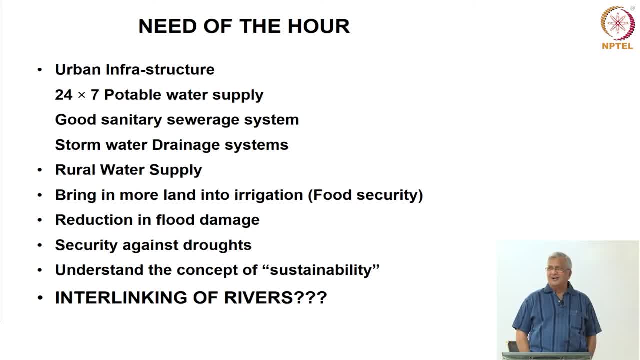 Kerala and Maharashtra and Karnataka and Bihar and Assam are going through floods and then of basically, excess water problem. in Chennai, we are desperately looking for one extra drop of water. We have water scarcity problem and these things happen and so at the same time you have floods. 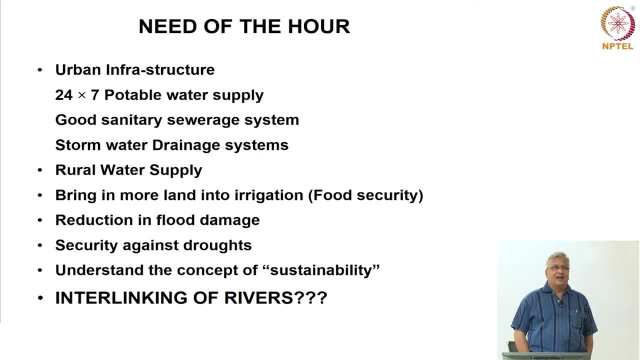 in one place and drought in the other place and in the same place. floods at one instance and drought in another instance. 2015, we had floods. 2016-17. we had severe drought already setting in Chennai. So how do we manage this water? 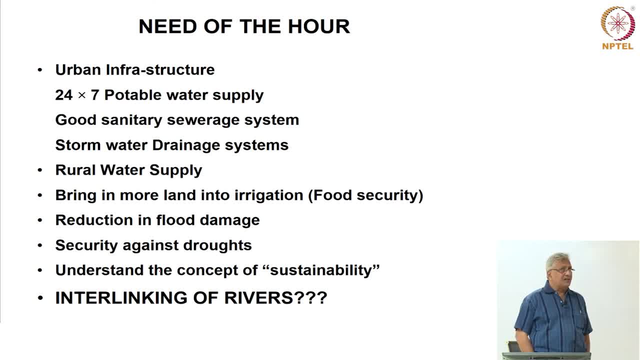 How do we manage the water between? agricultural sector, domestic water supply, industries also need water, and then we also have. sometimes we have too much of excess water. we don't know how to store it. we don't know how to use it for the future. we say that if we build 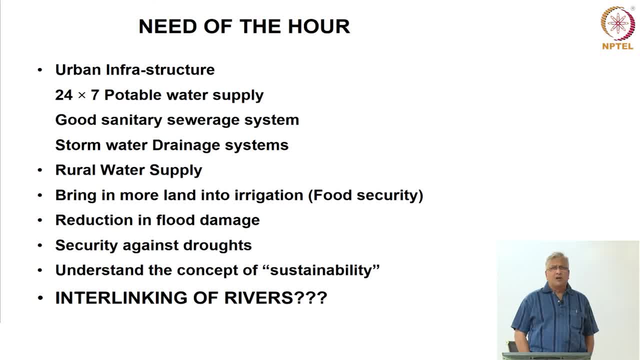 dams, then they have other environmental problems. all these things are completely interconnected and in fact one would like to connect up the entire infrastructure, let's say for urban infrastructure, sewerage system, storm water drainage system, water supply and you know, and even restoration of rivers, for nice waterfronts we need to have, because we also look at these. 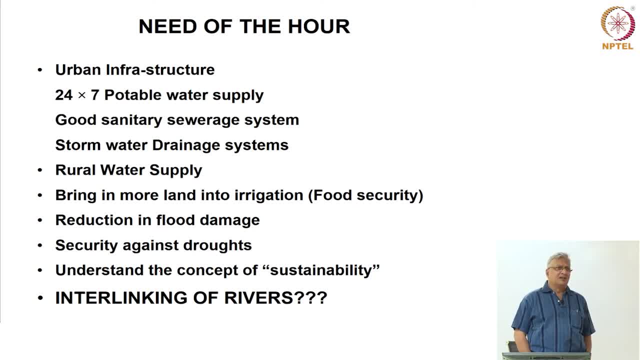 rivers for recreational purposes. That's what we are doing. Recently in Jaipur city. they have actually restored one particular small Dravyavati river, or they call it Amanisha Nala, which was in a dilapidated condition. they basically restored it because they wanted to have a nice riverfront through the city. 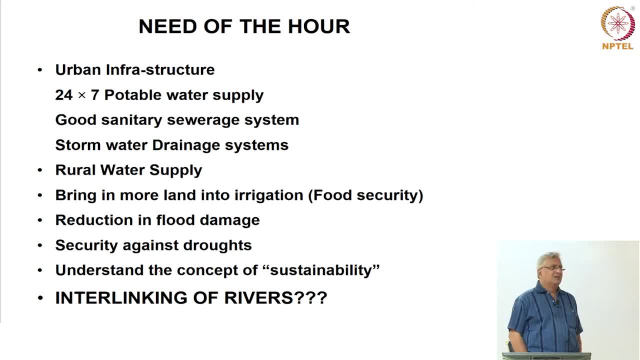 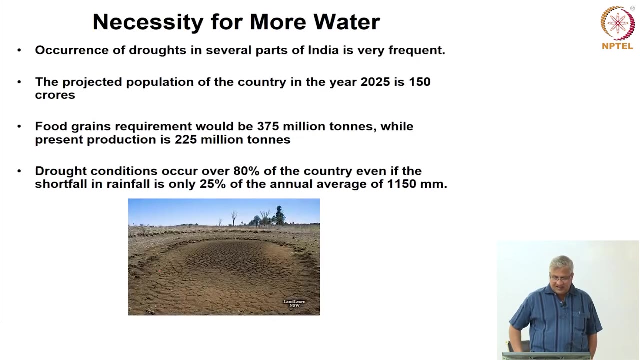 So all these activities should be looked at together simultaneously and design it so that you know in the long run they are all sustainable. So in this Context, in India they have been talking about interlinking of rivers, that is, inter basin transfer of water, basically the need I mean. in fact they have been talking about 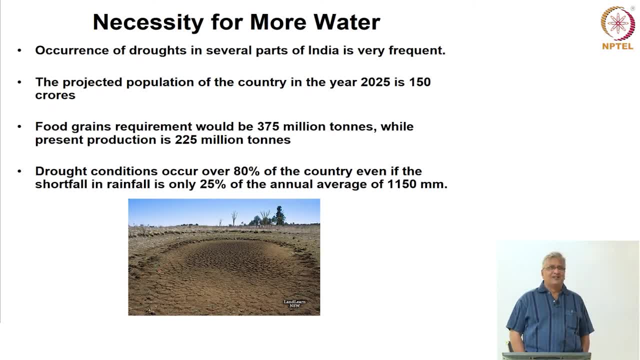 interlinking of rivers since 1960, we haven't yet implemented it, and the reasons why we did not implement and why we still discuss about it is becomes apparent when you see these points. We need the interlinking of rivers. the people who root for interlinking of rivers their 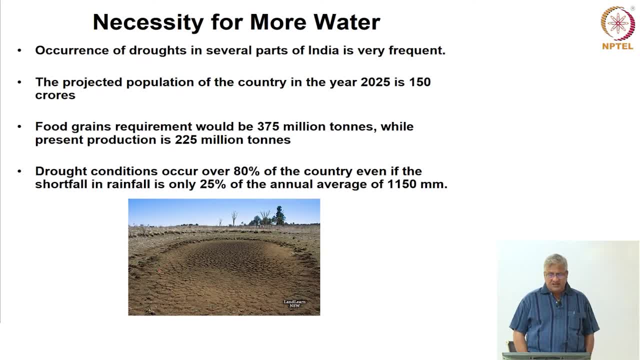 arguments are, of course, which are right. occurrence of droughts in several parts of in India is very frequent. like peninsular India, we have lots of droughts, and then western part of India also, we have lots of droughts. we don't have much of rain, we don't have much of water. 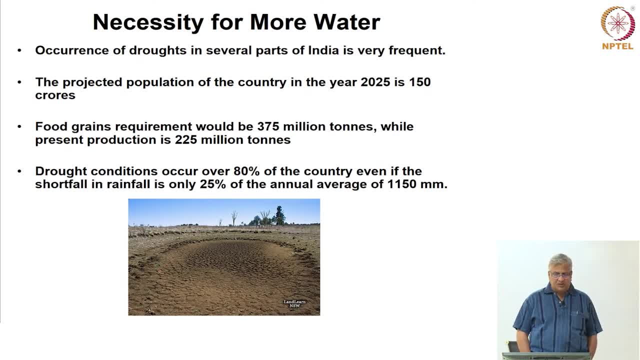 and projected population of the country is going to be 150 crores. So we have a lot of droughts, We don't have much of rain, we don't have much of water and projected population of the country is going to be 150 crores. 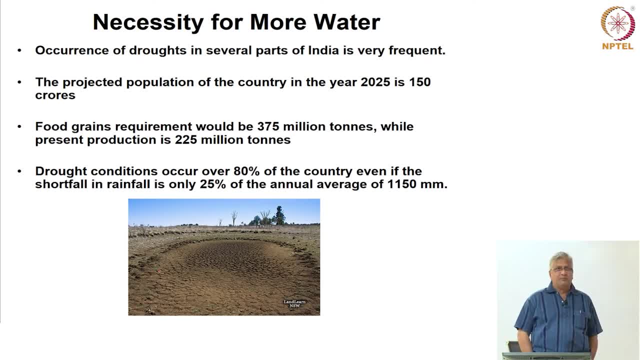 That is 1.5 billion, and we would be the most populous nation in the world soon. Food grains requirements would be 375 million tons, while the present is only 225 million tons. So you have to see how much of improvement we have to make in our agricultural sector. 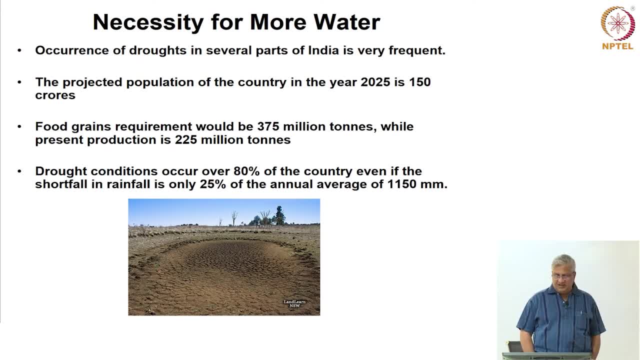 and droughts occur 80% of the country. in 80% of the country, even if rainfall is only 25% shortfall. There is only 25% shortfall in rainfall, then 80% of the country is under drought. So imagine what are the consequences of this. and then, at the same time, we have floods in. 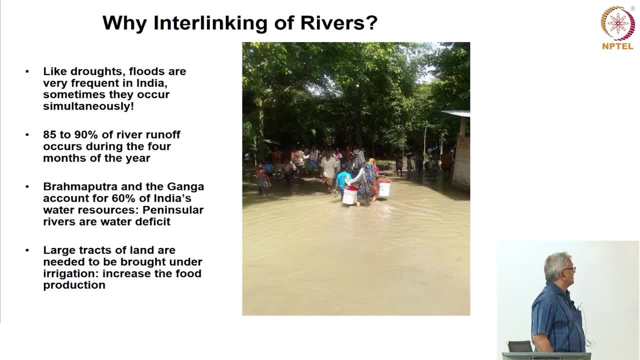 other parts, like droughts. floods are very frequent, they occur simultaneously and another important thing is because of the weather conditions. in India, 85 to 90% of the country is under drought, 90% of the entire what we call runoff. runoff is the water that is flowing in the rivers. 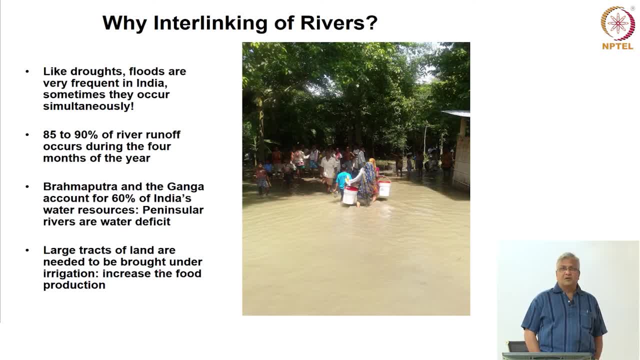 due to the rains. It occurs in the 4 months out of 12 months. only 4 months. you get the rainfall and 2 rivers. we have such a vast area and in that and so many rivers, only 2 rivers: Brahmaputra and Ganga. they account for 60% of India's water resources. 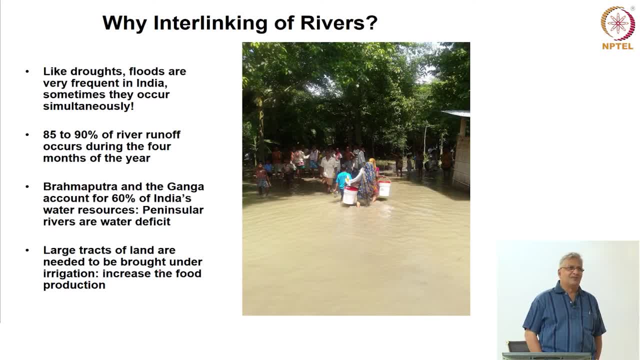 So this is the situation. Thank you, Thank you, Thank you. You have the coming three months and all these are going to extreme. Dropping losses has theplementations because YepNow, in this situation, the Odessa-Cライ. thank you for that. it is such a relief to be able to say if you are the 달라 working. 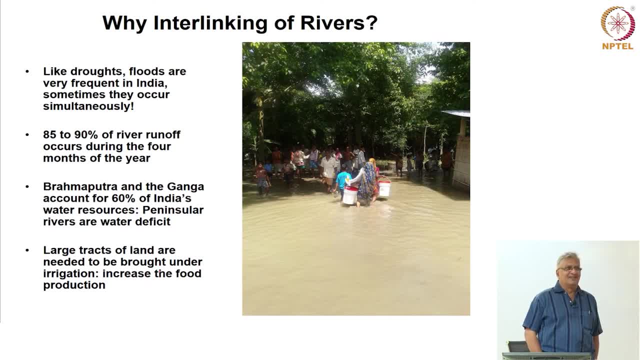 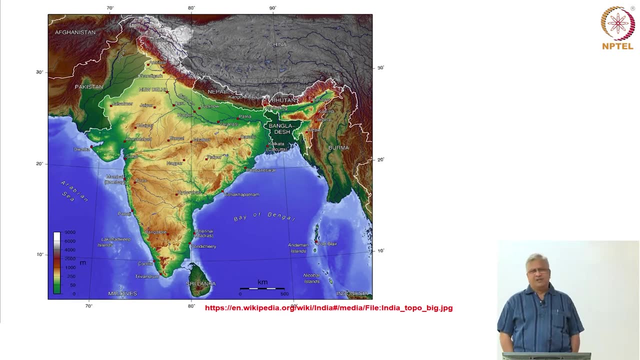 in the way in it And I, if anybody wants to say anything, go ahead. You're welcome. All have a good afternoon. All have a good afternoon. We will be no problem. Have a good afternoon, Thanks. already said so. they said: why don't we do a mega project? we have lot of water in Brahmaputra. 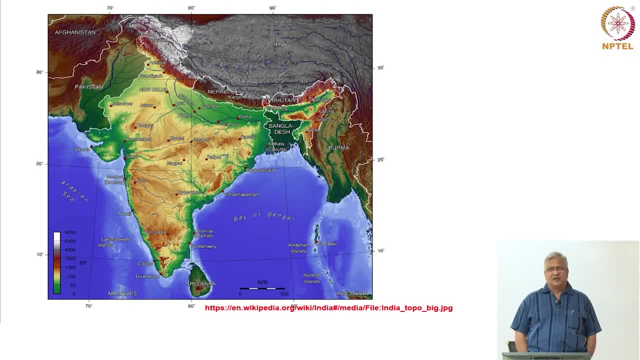 and then this lot of water is, of course, causing lot of floods in the downstream areas in Assam as well as in Bangladesh. so why don't we divert this water from Brahmaputra and probably put it in Ganga? you build a huge canal and then put it in Ganga, and we have now excess. 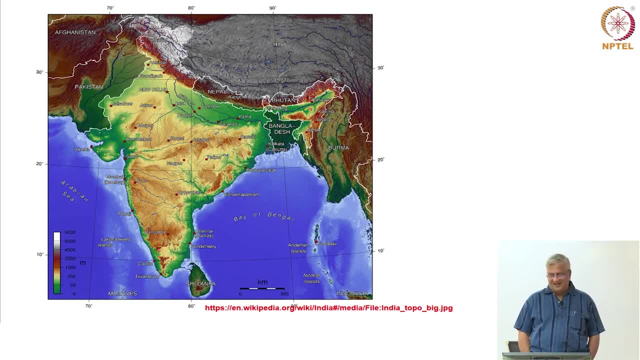 water in Ganga. so you take water from Ganga and you cross Subadnarekha in border of Orissa and Bengal and then get down to Orissa and then put it in Mahanadi. now, from Mahanadi you go and take it to put it in Godavari, and from Godavari you put it in Krishna, from. 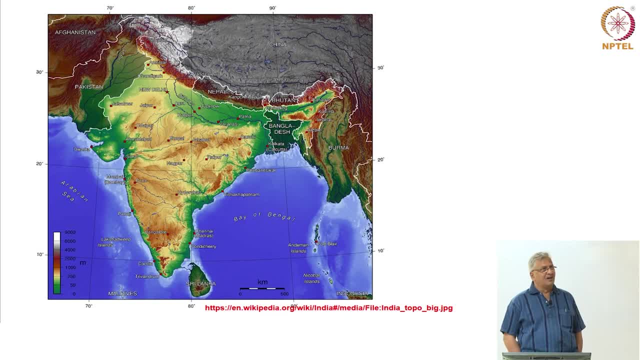 Krishna, you can put it in: you know, Penna river, And then from there to Kaveri and then all the way down some other rivers, So you can redistribute the water wealth for the entire country by putting this so called and of course in the North Indian rivers many other rivers also. they have linking of. 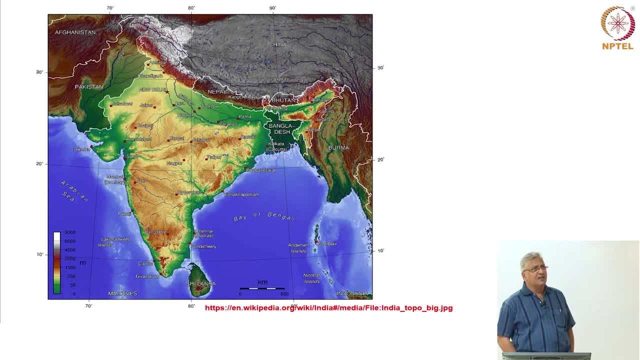 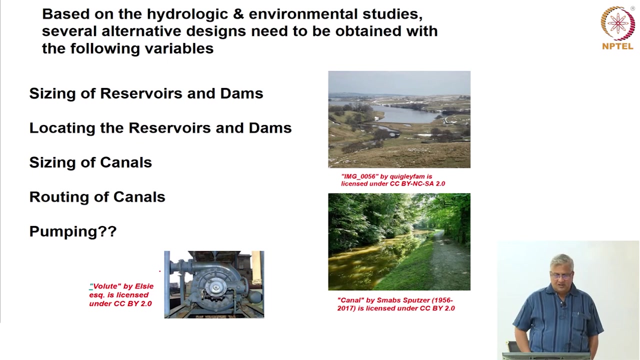 these rivers, small, small rivers, so that there is a redistribution of water for the entire country, and then probably we will be able to solve our food problem And all the other water problem. very nice idea, but the issue is: what are the constraints? 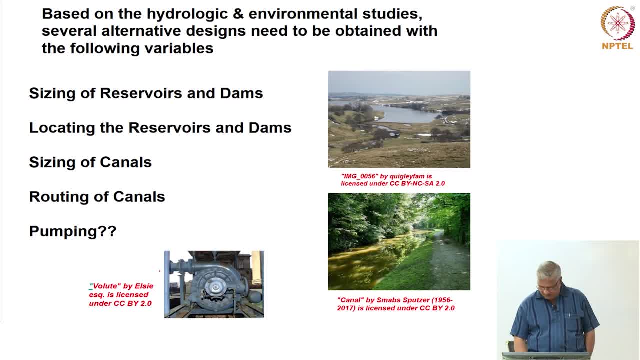 these are before we go to the constraints we will discuss about. as hydraulic and water resources engineers, we have to conduct hydrologic and environmental studies and we have to come up with several alternative designs. Thank you means basically, we should define our goal and then we should say that like this particular. 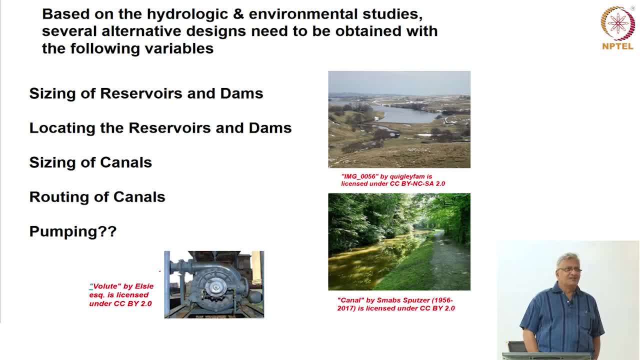 project is the only way that we can solve these problems or attain these goals. and as engineers, we say: what are the things that we can contribute? what should be the size of the reservoir? what should be the size of the dam? this, of course, depends upon how. 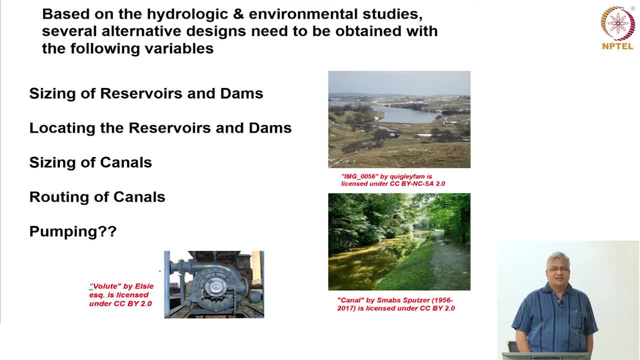 much of water is coming in. in that, let us say Mahanadi. we say I want to build a new dam. so I ask: what should be the size of the dam? what should be the size of the reservoir? this depends upon how much of water is coming in. it depends upon how much is already being. 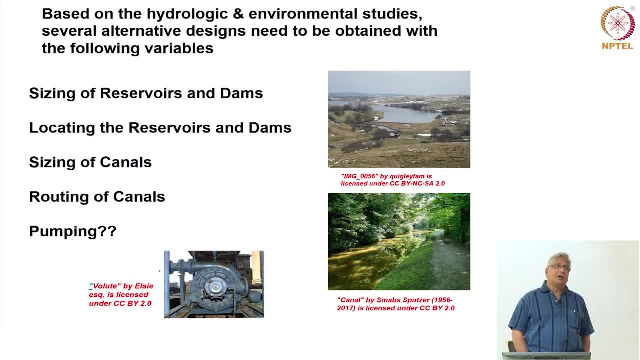 utilized there. it will also depend upon how much those people are planning to utilize in the future. you say that, like you know, I will take the water. probably people from Odisha are saying I may not be using all this water, so you may be thinking that I am wasting the water. 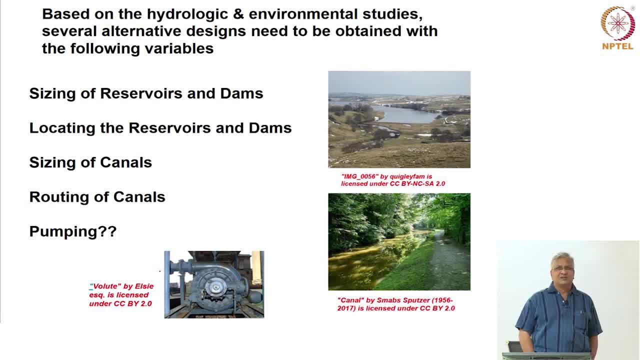 but I have so many other projects in my mind which I would use them in 2050, so I do not want to give you the water. they can say that and they have every right to say that. So, sizing of reservoirs and dams: that is where you need to do hydrologic studies as well. 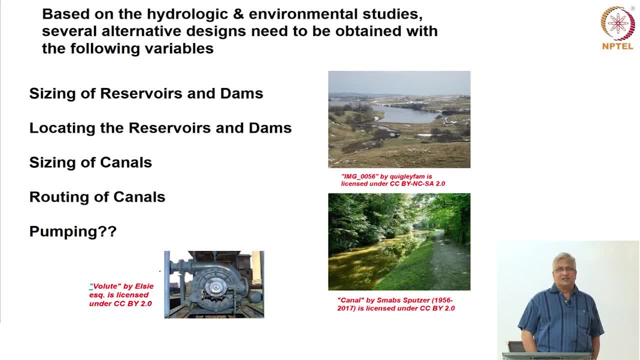 as hydraulic studies. then where do you locate these reservoirs and dams? what is the best location for these things? We have to do that, then, from one dam to another dam, which is on the downstream side. you have to connect up using canals. so how, what should be the size of the canals and what should? 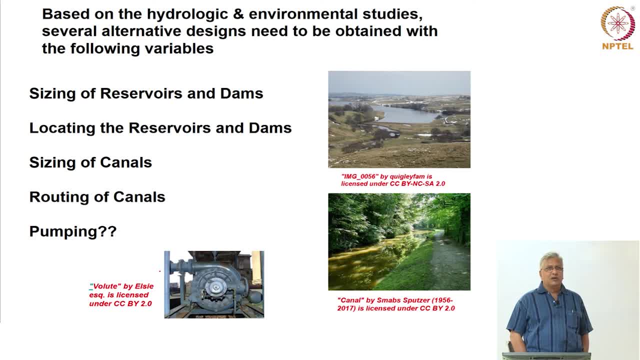 be the routing of canals. how do I route this? Because when I connect up from Mahanadi to Godavari, if I go, take all the way through east coast, then you have many east coast rivers which are flowing into Bay of Bengal and you 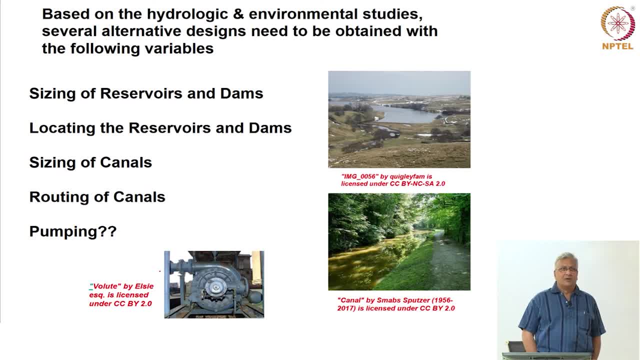 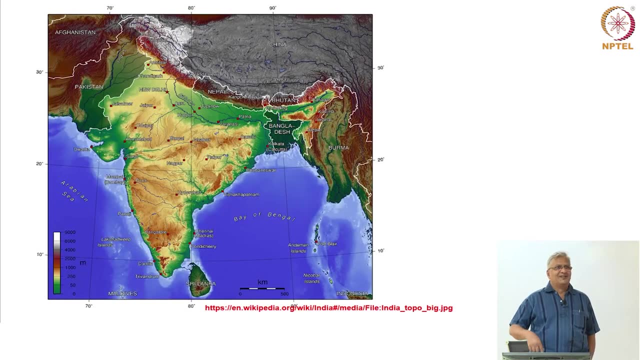 have to cross These rivers and you have lot of, you know, urban centers. you have to go, take it through the urban centers. How do you do this routing of canals? then, just because I put the map, Indian map from like this, I draw one link from north to south, does not mean that the water will flow down. 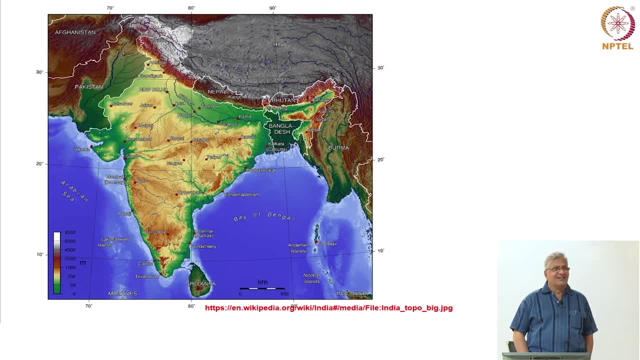 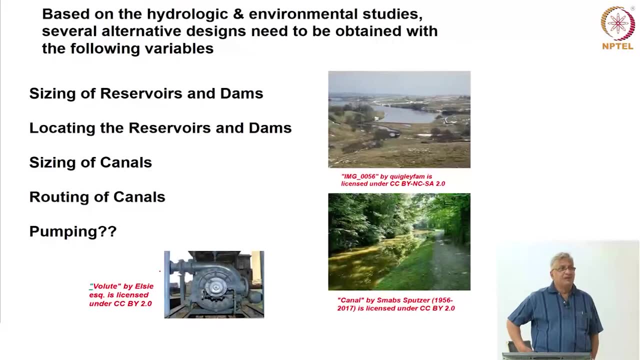 south. it all depends upon topographical conditions. we have the levels, we have ground levels, we have, and so on and so forth. So sometimes we may like, for example, if I want to take from Ganga to Narmada and then below to all those things, if I want to take that route, then I have Satpuras and Vindhyas. 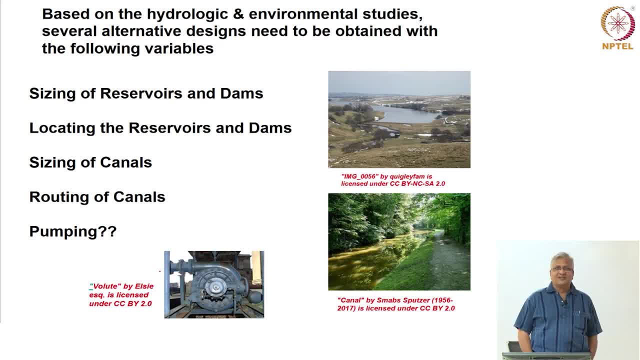 coming in between. So how do you cross them? you want to put tunnels, or you want to go and then put pumps. so many times you may need to pump water from one basin to another. Then in that case, what should be the size of the pumps? that becomes an important question. 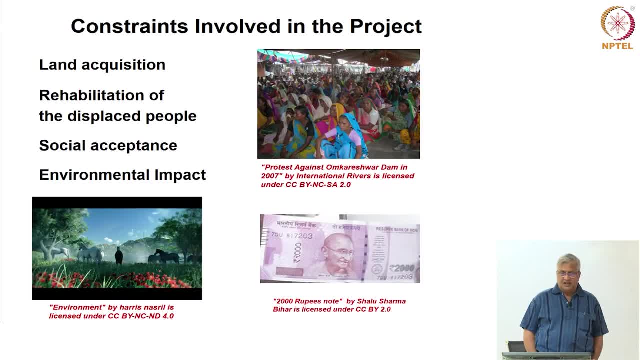 that I think water resources engineers would like to answer. This is one issue- the engineering issues- but we cannot run away from the other issues because constraints are: you need land and land acquisition. We were working with the Kerala government back in 2016 and so, and we came up with one. 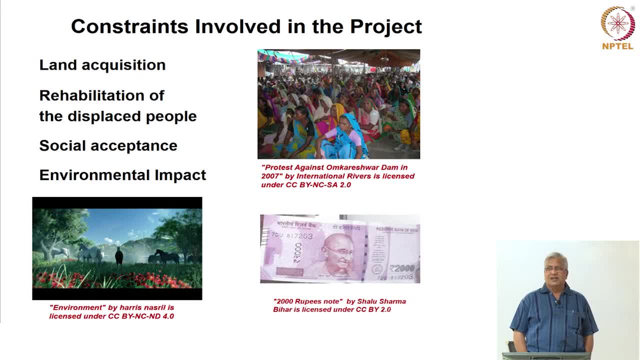 alternative. They started bringing in a system where they say, well, that is the way you can do the work, that you can do, that is the way you can do the work, But in most cases you have to do it in one basin. So they are really saying that, like you know, there is a link canal which takes the water. 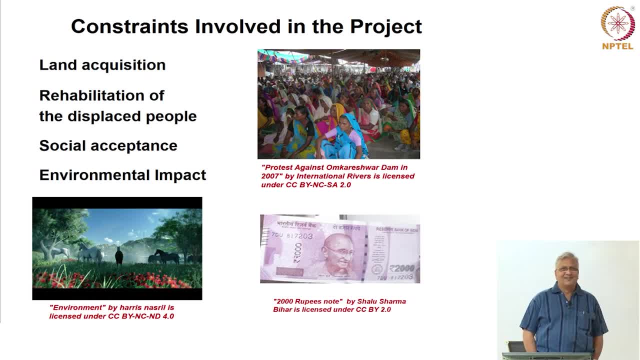 from one of the rivers to the Arabian Sea. We said: why don't you just increase the width of this link canal to maybe 300 meters- and we were asking only for about 20 kilometer stretch of this canal and then to 300 meters and then probably we can divert lot of this flood waters and then we can in Kootenai area. 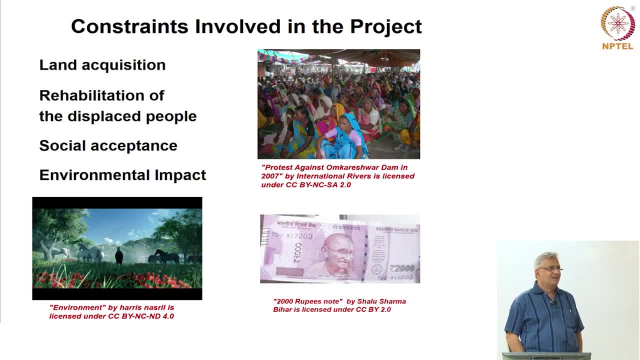 we can solve the flood problem. We gave that idea And then very nice, And in fact it is very nice. And the other thing I wanted to mention is the Amrit of the Kerala River. the Kerala River- It was a meeting with chief ministers and then all the technocrats and everybody. 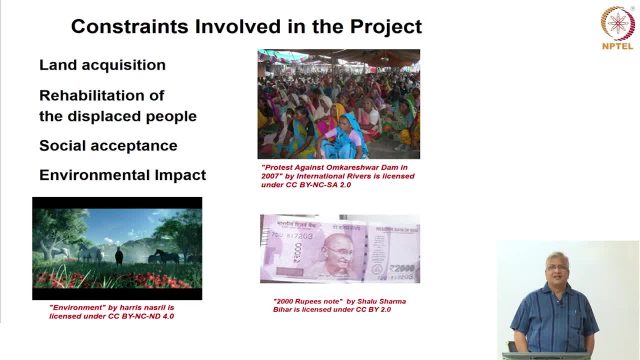 They said: very nice idea, but we cannot go and implement because we will never be able to acquire land in Kerala Because land is very, very costly. They won't sell the land, So land acquisition is a problem. Then another is rehabilitation of the displaced people. 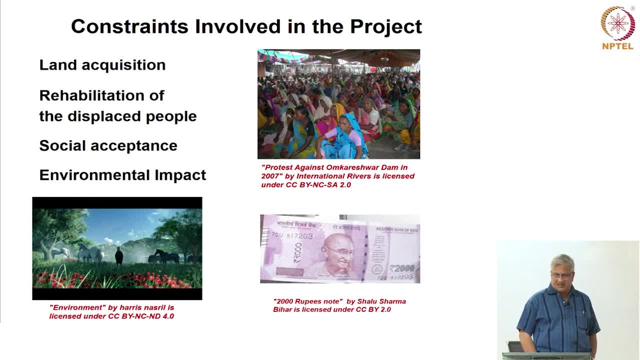 That's also a you see that picture that I have given. It's basically there's a protest against Omka Resho Dam on Narmada River in 2007 by local people. They would get displaced when you put these reservoirs and dams. 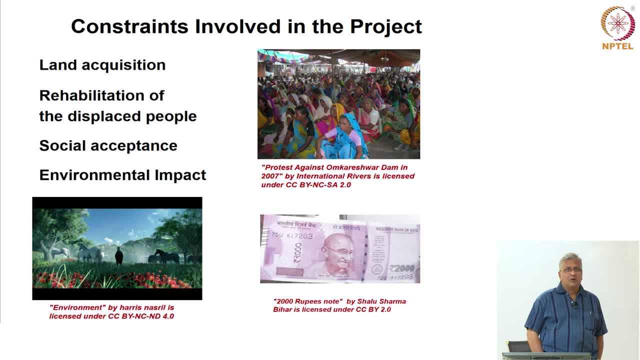 So they would protest. So what do you do for them? How do we make these projects socially acceptable is a very important issue. In fact, there is a new field of research, a new field of water resources engineering. It's called social hydrology. 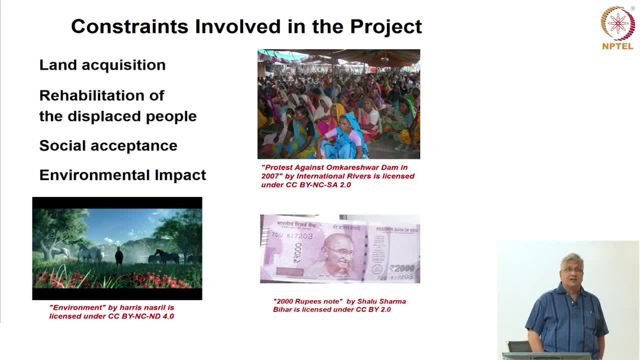 So how the hydrology actually gets affected by the response of the society and how we should take care of societal responses to our projects. Social hydrology is very important, And then we also need to think about environmental impact that this humongous project.